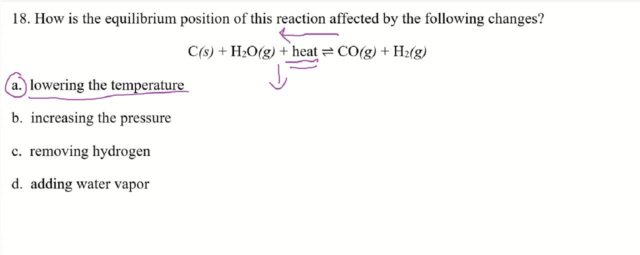 In other words, it's going to favor the reactants because it's going to try to undo that change that you just did to the system. All right, so this lowering the temperature is going to favor the reactants. Okay, let's go to. let's go to part B. 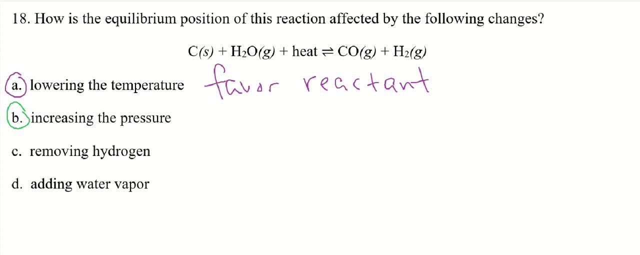 What happens if we increase the pressure of the system. So this is a system possibly in a, in a, in a container, And pressure is caused by the collisions of gas Particles with the walls of the container. So this only applies to gas particles. 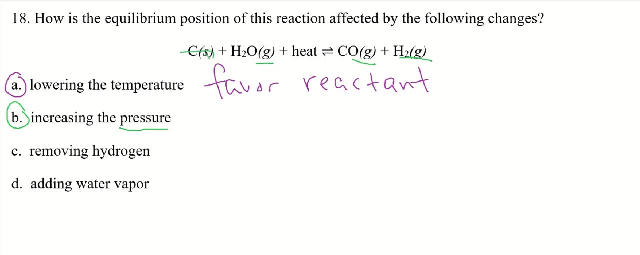 All right, so we're going to disregard this carbon because it's a solid It's. the pressure that it adds is negligible. So which side- the reactants or the products- has more moles or molecules of gases? All right, so here, on the reactant side, we only have one mole of water. 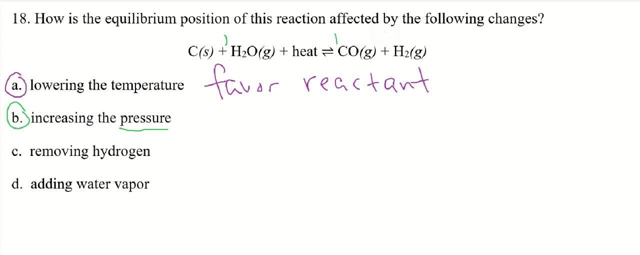 All right, and that's going to produce one mole of carbon monoxide and one mole of hydrogen gas. So we have two: two moles on the product side versus the one on the reactant side of gases, Right? so if we increase the pressure, how can the system relieve that pressure or decrease the pressure? 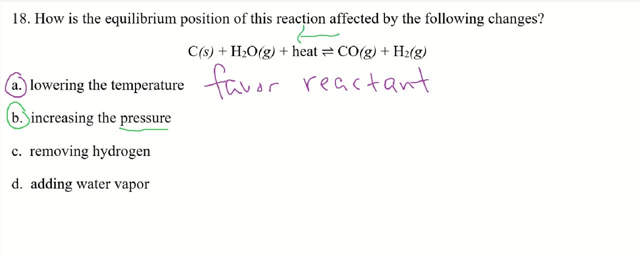 It's going to favor the side that has fewer molecules, gas molecules- So again, it's going to favor the reactants. Okay, part C: What happens if we remove hydrogen or we decrease? what do I do here If we? let me erase this from previous. 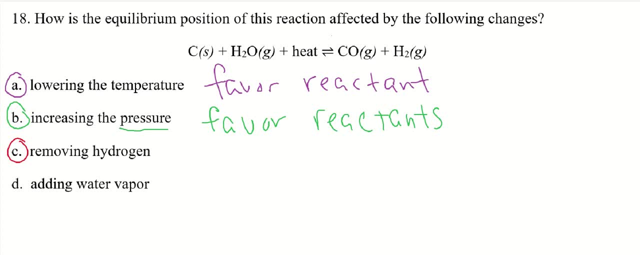 All right. what happens if we decrease the amount of hydrogen? Hydrogen is a product, Oops, sorry, pen. Hydrogen is a product. So if you remove a product, a system that was at equilibrium will try to create more of the product that you removed.